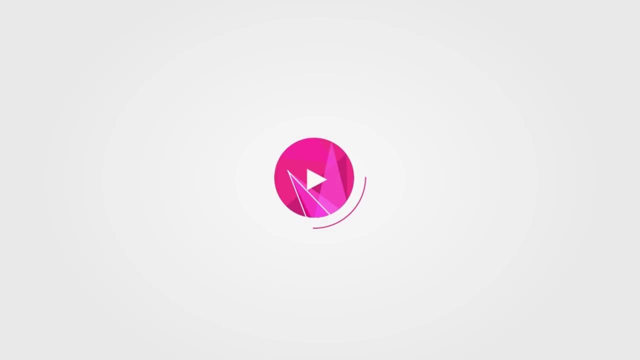 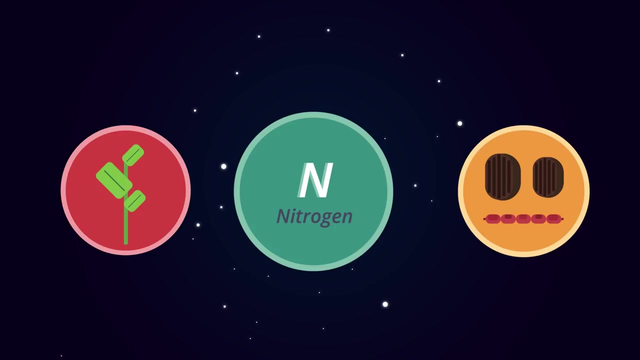 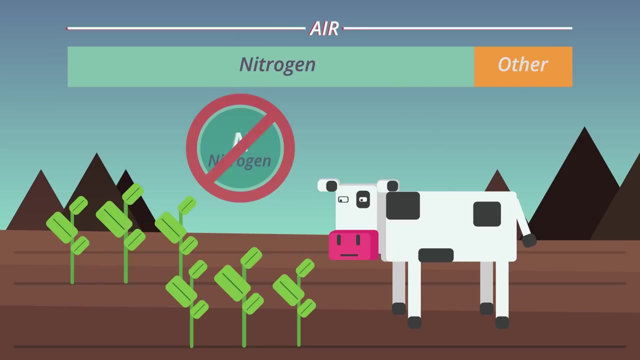 Nitrogen is essential to life. Plants and animals need nitrogen to make proteins, And proteins are the building blocks of cells and their full life. Nitrogen makes up 78% of the air. however, neither plants nor animals can take nitrogen directly from the air because nitrogen is so unreactive. 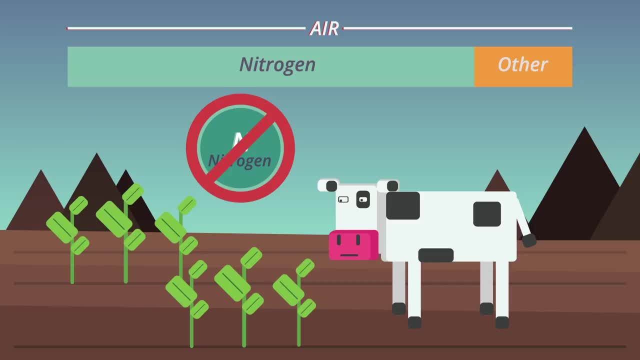 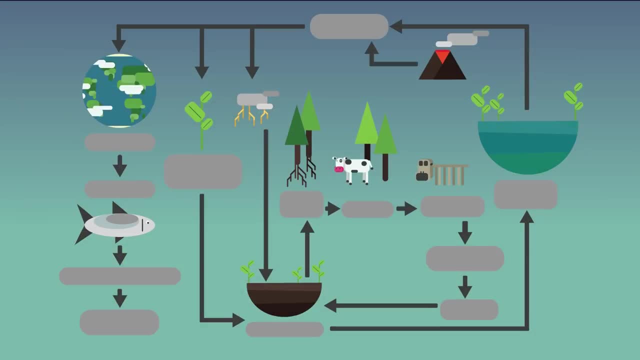 However, plants are able to take nitrogen compounds, such as nitrates, from the soil, And then animals eat these plants, therefore providing animals with a source of nitrogen. In this video, we are going to look at the nitrogen cycle. This is the movement of nitrogen through the environment. 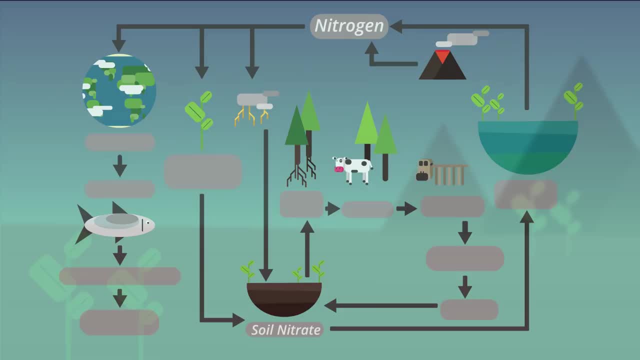 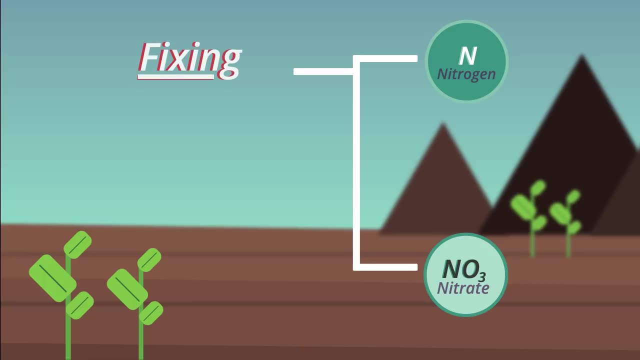 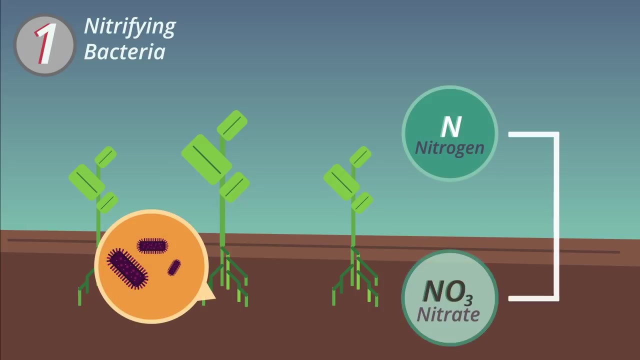 Nitrogen is continually cycled through the air, soil and living things. The process of nitrogen in the atmosphere being turned into nitrogen in the soils is called fixing. Here are four different ways in which nitrogen fixing occurs naturally. Firstly, nitrogen fixing bacteria in the soil turns nitrogen from the air into nitrates, which the plants can then absorb. 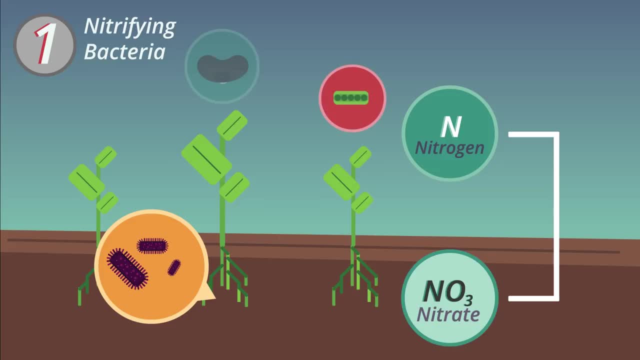 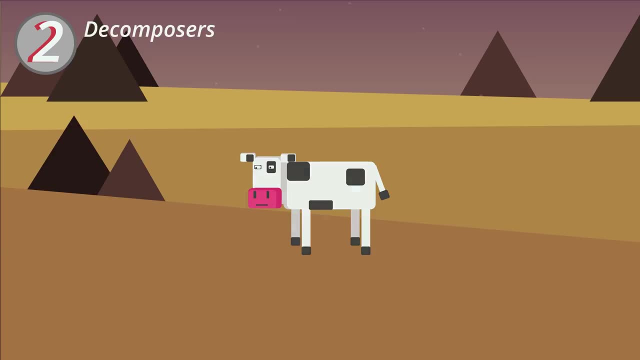 Some plants, such as the legume family, which includes peas, beans and clover, have these nitrogen fixing bacteria in their root nodules. Secondly, decomposers in the soils break down animal excretion and dead organisms, returning nitrogen back to the soil as ammonia. 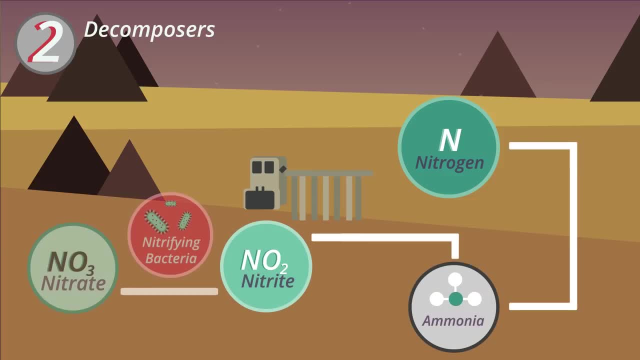 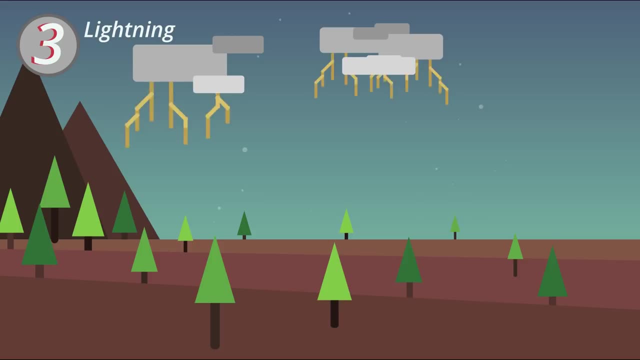 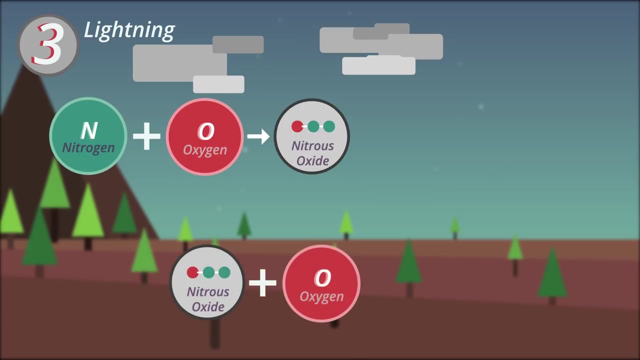 The ammonia turns firstly into nitrite and then nitrifying bacteria in the soils turns the nitrite into nitrate. Thirdly, lightning can cause chemical reactions in the atmosphere, resulting in nitrogen reacting with oxygen to produce nitrous oxide. The nitrous oxide then reacts with more oxygen and dissolves in rainwater to make nitrous acid. 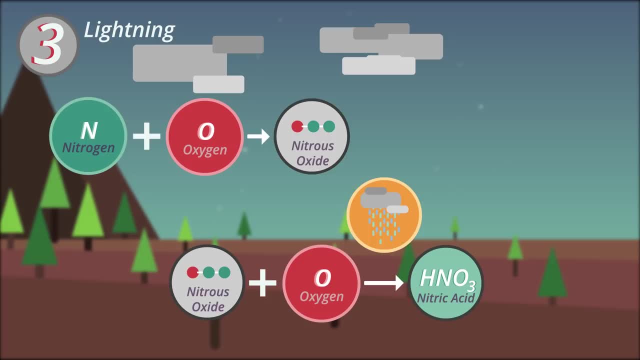 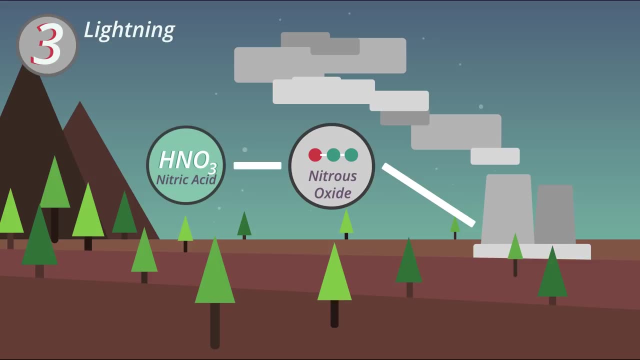 This rainwater containing nitrous acid increases the amount of nitrate in the soil. Burning fossil fuels also adds nitrous oxide to the atmosphere, resulting in nitric acid, But this is, of course, not a natural way of nitrogen fixing. And finally, in the oceans, many species of blue-eyes appear. 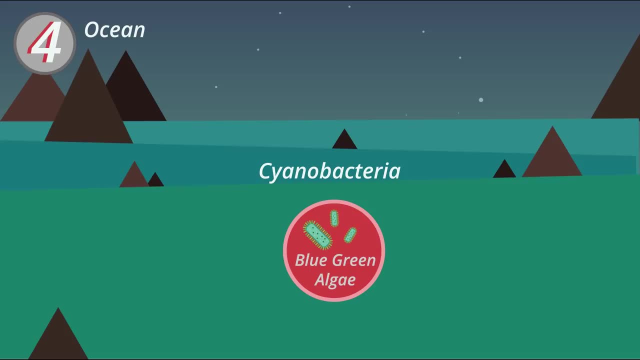 And finally, in the oceans, many species of blue-eyes appear. The blue-green algae, also called cyanobacteria, can fix nitrogen. This then provides sources of nitrogen to aquatic animals And the nitrogen goes around, a similar cycle to what happens on land. 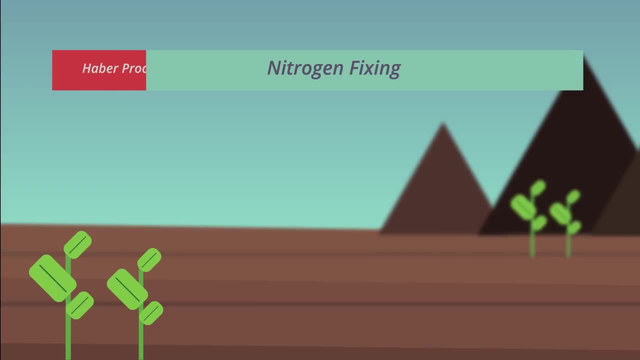 These are the natural ways through which nitrogen fixing occurs. The harbour process, which is how fertilisers are made, makes up approximately 30% of the nitrogen fixing, Because nitrogen is essential for making proteins. proteins are essential for cell production. Cell production is how growth occurs.